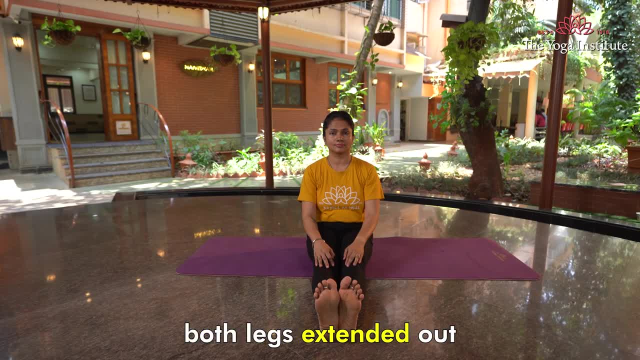 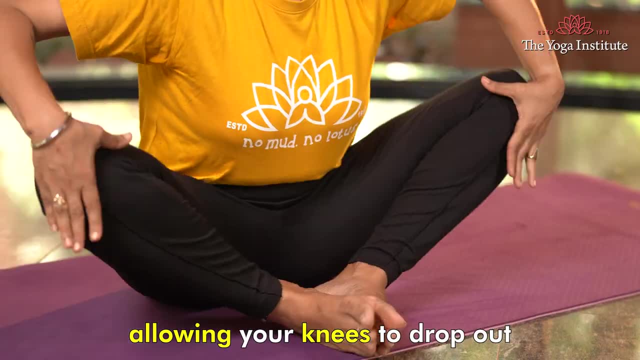 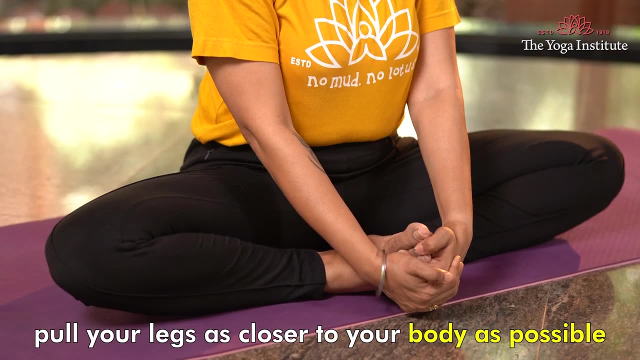 let's look at Bhadrasana. Begin seated with your both legs extended out in front of you. Bend your knees and bring the soles of feet together, allowing your knees to drop out on the respective side. Hold on to your ankles with your hands. Pull your legs as closer to. 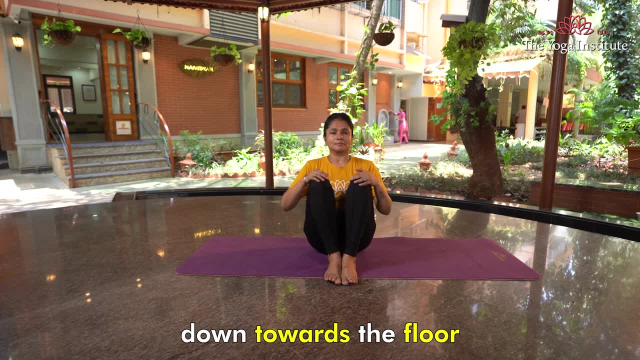 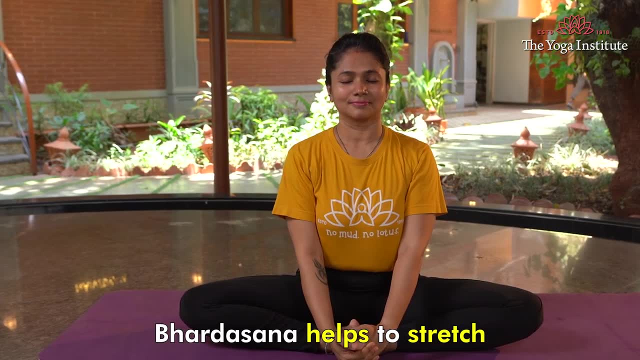 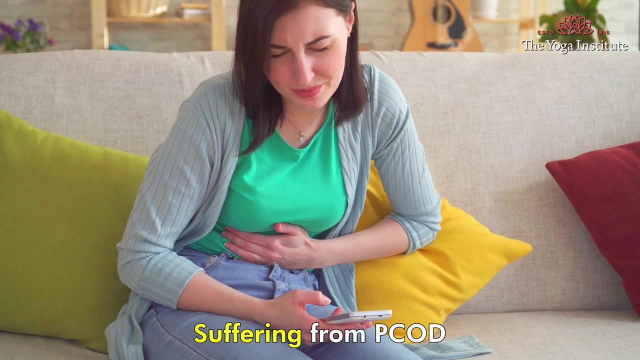 your body as possible and press your knees down towards the floor. Hold for some time and then release. Do this for a few rounds. Bhadrasana helps to stretch and open hips and groins, which can be helpful for the woman suffering from PCOD. 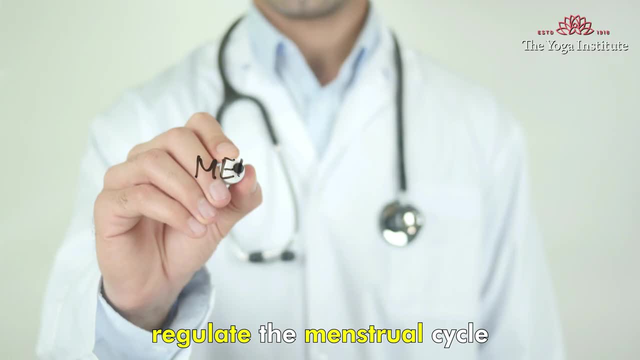 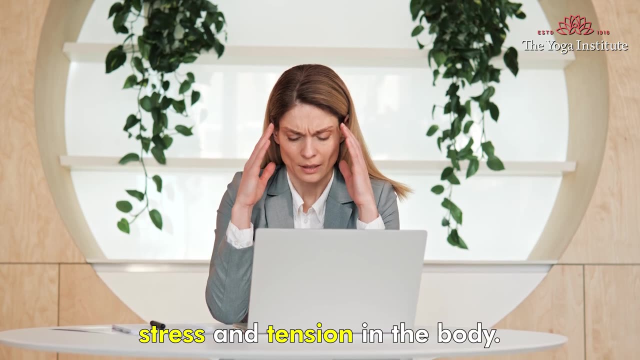 The circulation to the pelvic area, which can help regulate the menstrual cycle and reduce menstrual cramps. It also releases stress and tension in the body. Next is Paryankasana. Sit down in Bhadrasana, Spread your feet apart. 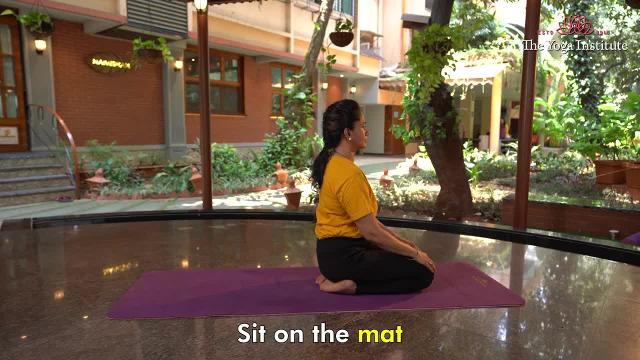 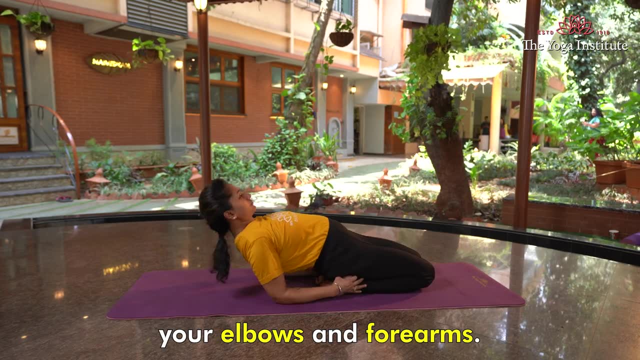 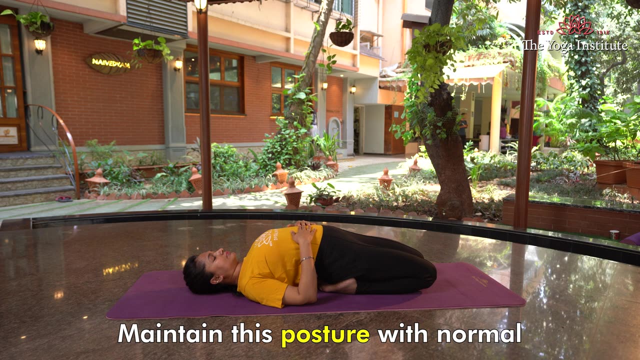 trying to keep your knees together. Sit on the mat in the space created between your feet. Lean backward with the help of your elbows and forearms to lie supine. Interlace your fingers and hold your hands over your abdomen. Mental position: with normal. 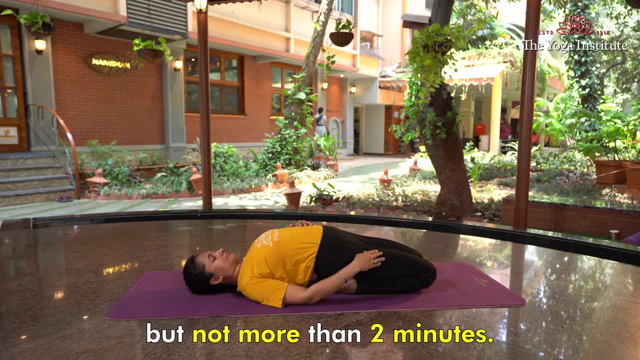 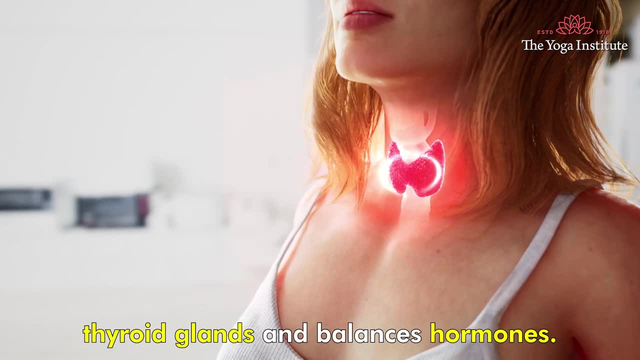 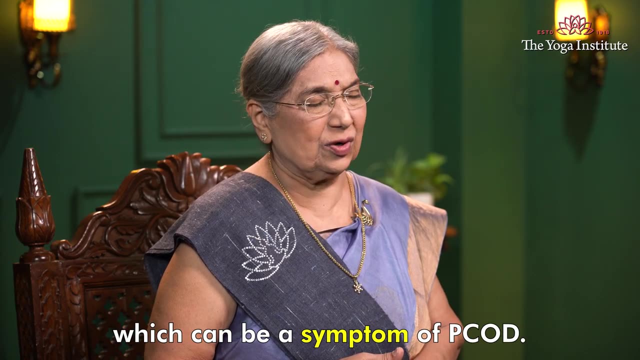 rhythmic breathing. Stay comfortable, but not more than 2 minutes. Next is Paryankasana. Paryankasana helps to regulate the thyroid gland and balances hormones. Paryankasana improves digestion and releases constipation, which can be a symptom of PCOD. It releases stress and anxiety. Stress and anxiety. 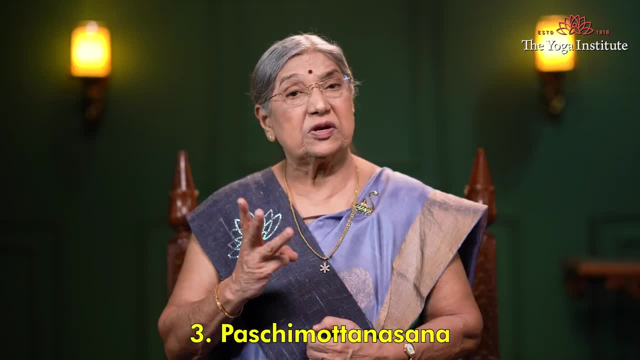 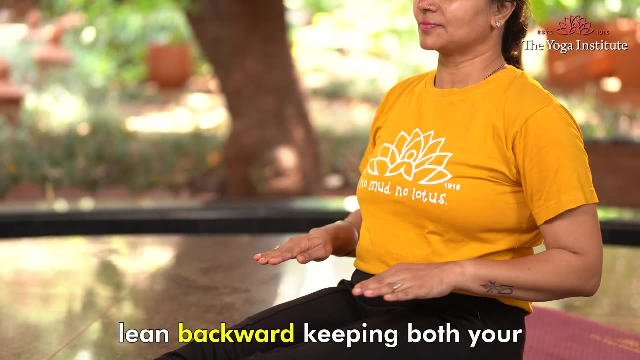 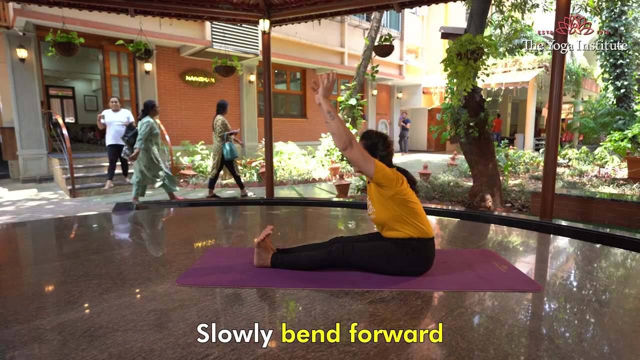 worsen the condition of PCOD 3. Pashimottanasana. Sit on the floor with legs extended in front of you, lean backward, keeping both your palms facing downwards and, besides, chest hands folded at the elbow slowly bend forward. 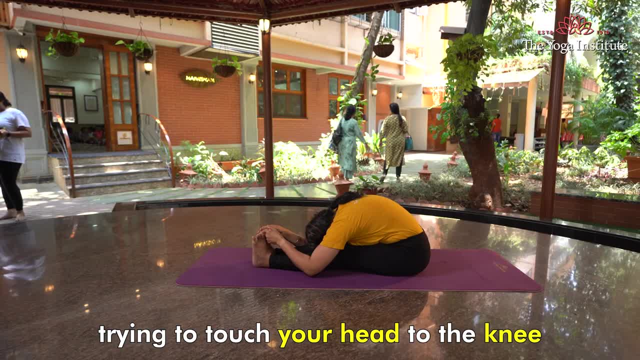 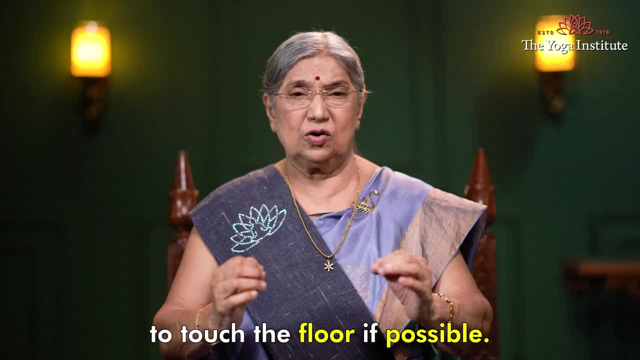 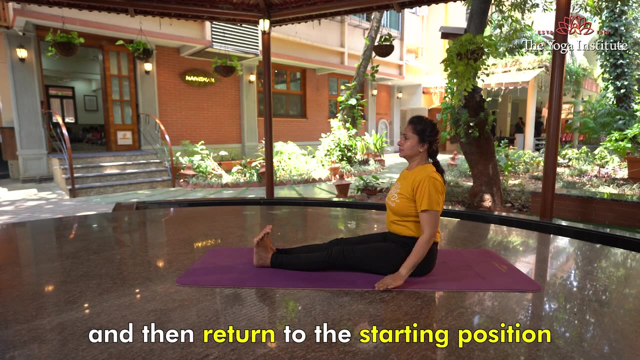 stretching your hands to hold your toe, trying to touch your head to the knee without bending your knee here. you can even try to lower your elbows to touch the floor, if possible. Remain in this position for few seconds and then return to the starting position. 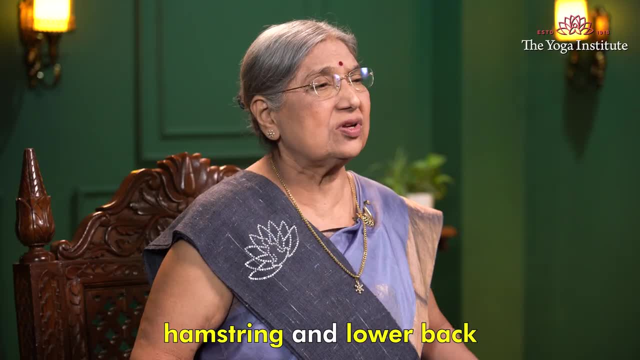 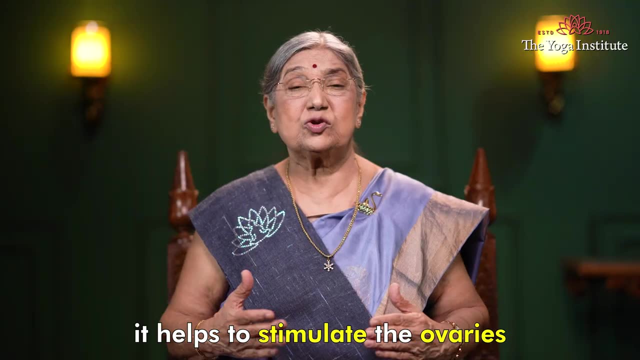 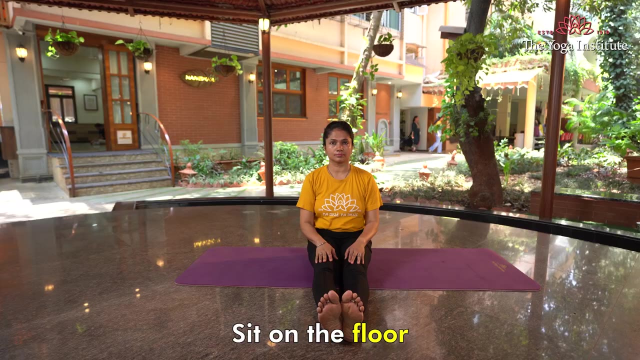 Pashimottanasana stretches your spine, hamstring and lower back, which can reduce back pain and discomfort that may come with PCOD. It helps to stimulate the ovaries and improve hormonal balance. 4: Ardhamatsendrasana: Sit on the floor with both the legs extended in front of you. fold your right leg inwards. 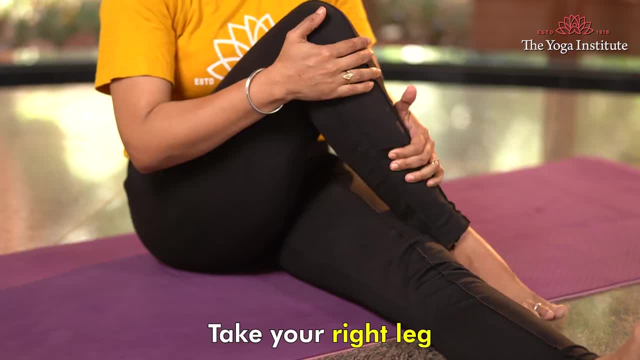 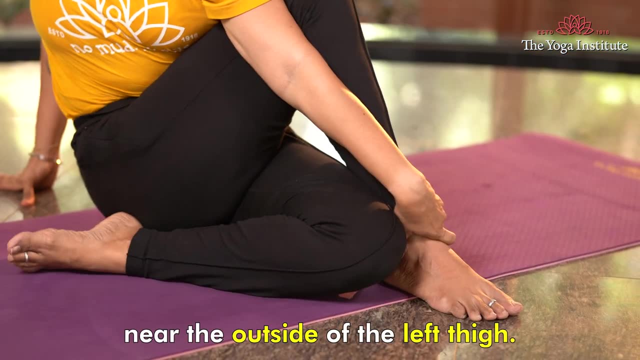 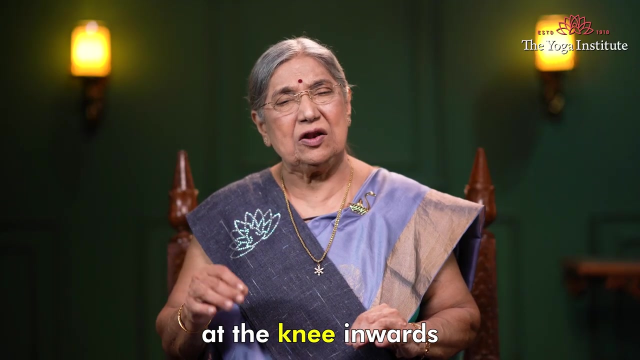 and bend your right leg inwards. Press your heel against the perineum. Take your right leg bending at the knee, crossing across your left thigh. Place your right foot near the outside of the left thigh and bring your right knee close to your chest. Bend the left leg at the knee inwards and place 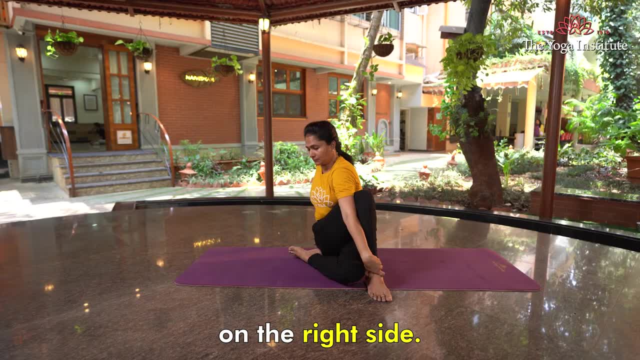 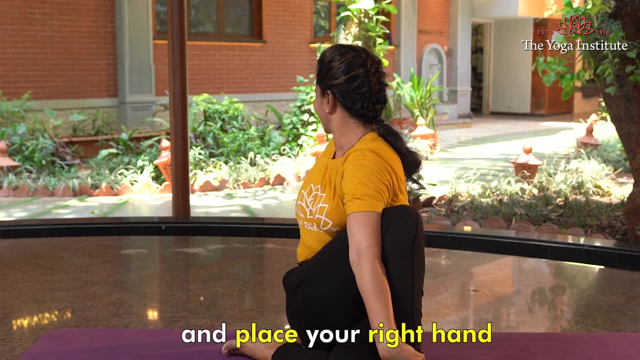 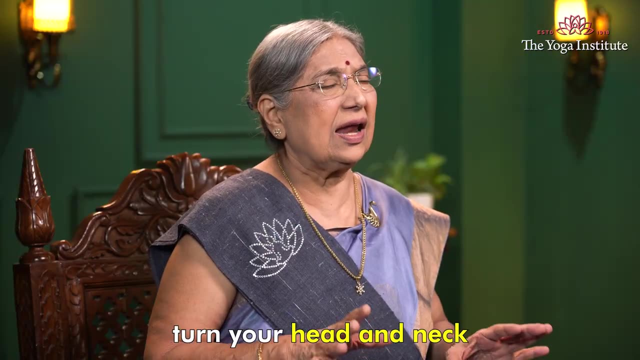 your foot close to your right hip. Twist your torso on the right side, Let your left hand hold your right ankle or toe. Give more twist to your spine and place your right hand across your back with the palm facing outwards. At the same time, turn your head. 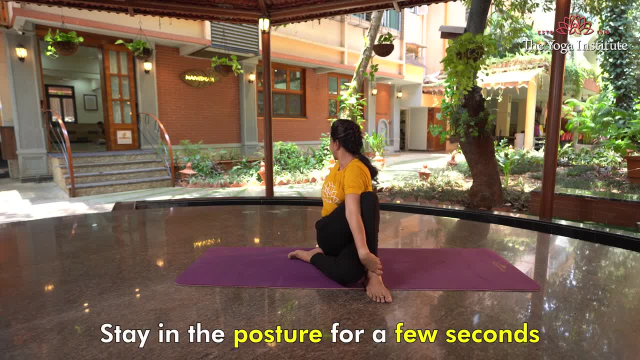 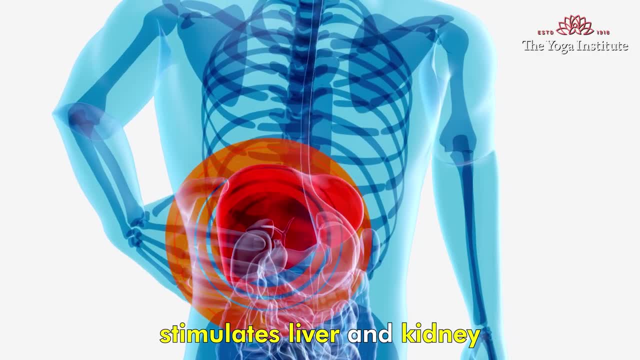 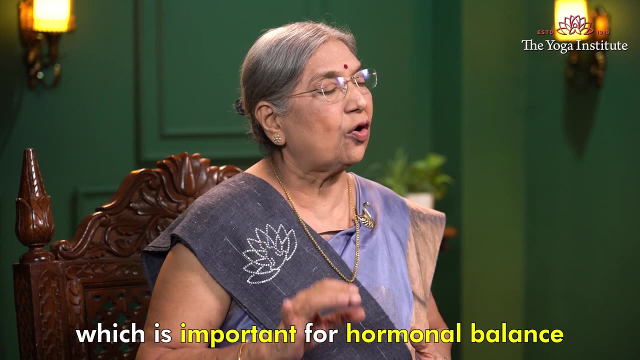 and neck towards your right shoulder. Stay in the posture for few seconds and then come back to the starting position. 5. Ardhamatsendrasana Stimulates liver and kidney, which can help detoxify the body and improve liver function, which is important for hormonal balance. It stretches the shoulder, hips and spine, which can 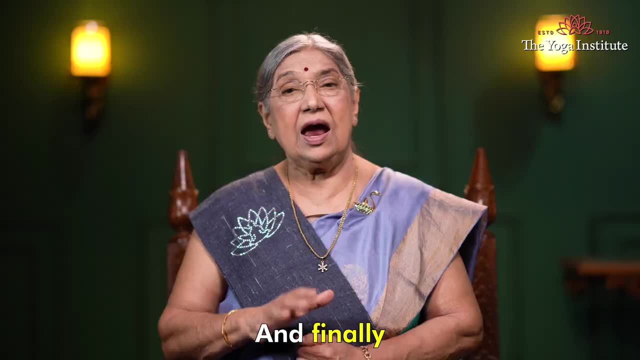 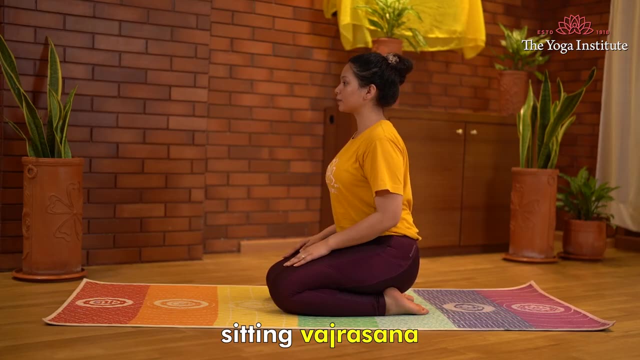 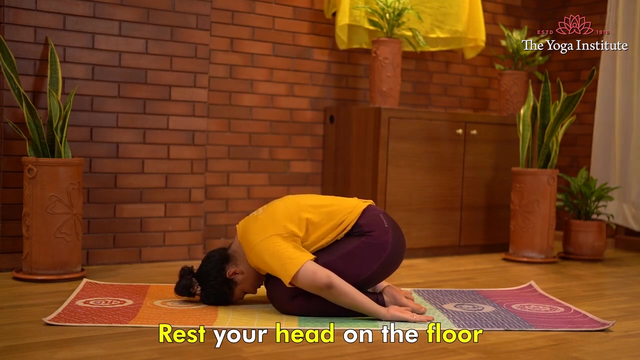 alleviate tension and discomfort in those areas. And finally, now we have forward bending asana, and that is Balasana. Sit in Vajrasana, Slowly bend forward, keeping your hands by your side, palms facing up. Rest your head on the floor, if possible for few seconds, and then return to the 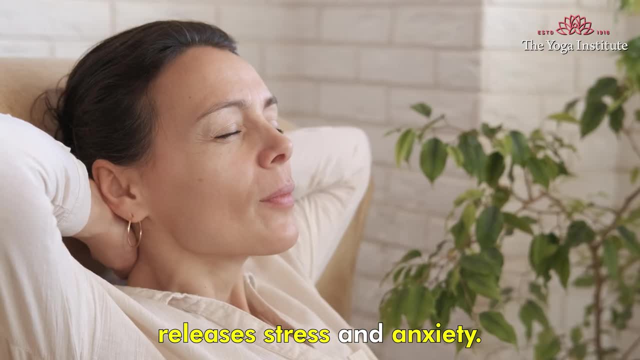 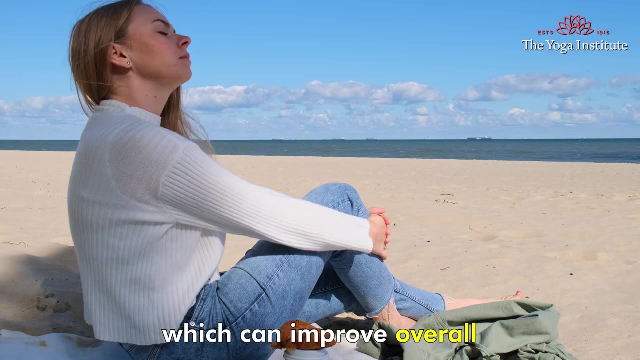 starting position. Balasana calms the mind, releases stress and anxiety. It helps to improve blood flow to the next stage 7, Balasana. The Balasana is a very effective yoga asana to the reproductive organs which can improve overall. 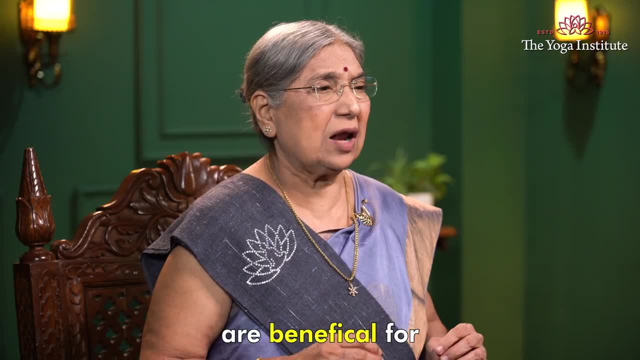 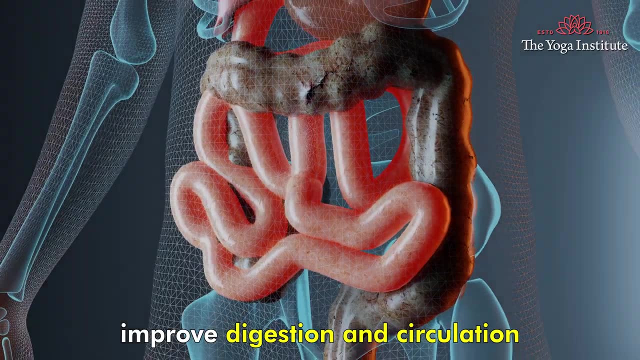 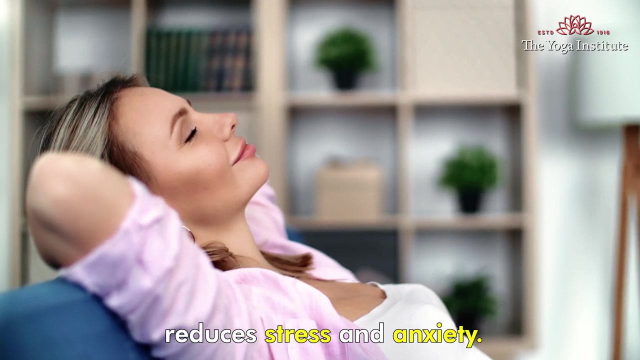 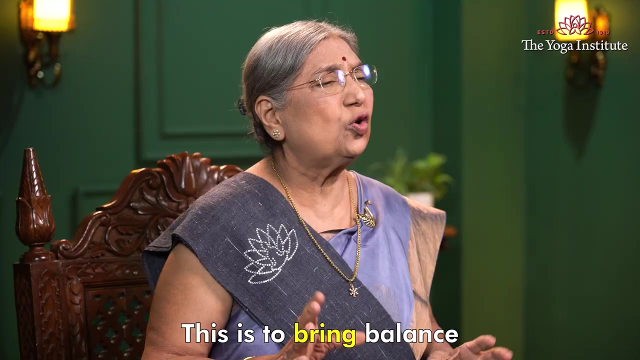 reproductive health. These five yoga asanas are beneficial for women for PCOD, because they help to regulate hormones, improve digestion and circulation, elevate pain and discomfort and, above all, reduces stress and anxiety. Learn and practice these asanas to manage PCOD disease. to.